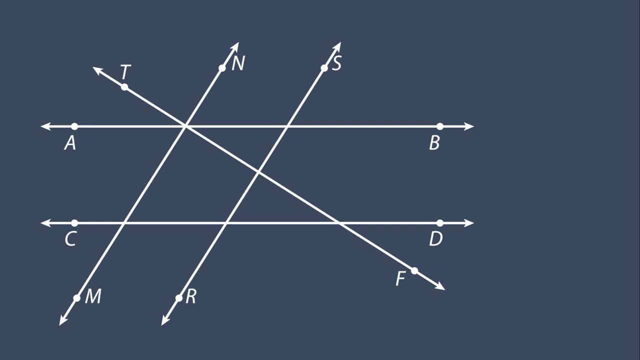 and the pairs of lines that appear to be perpendicular. Let's start with the parallel lines. Remember that parallel lines have to be the same distance away from each other and parallel lines never intersect. From this model, we can see that line AB is parallel to line CD. 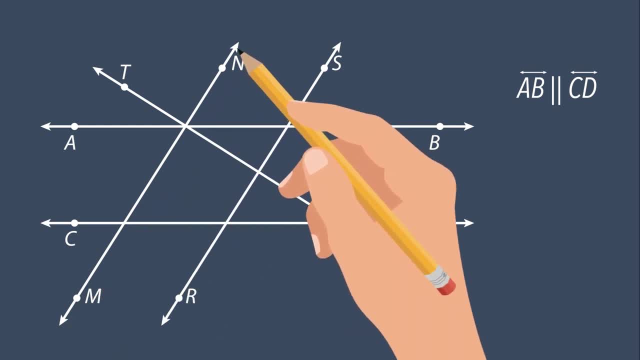 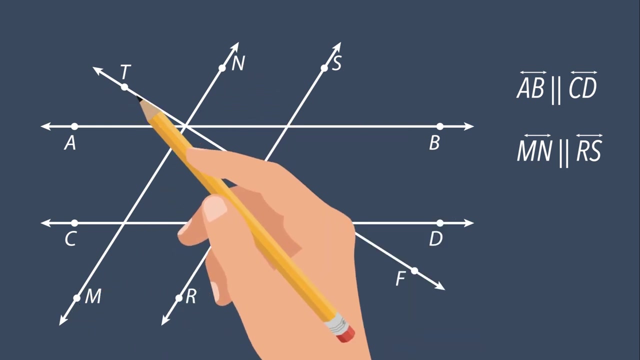 We also notice that line MN is parallel to line RS. Now let's look for perpendicular lines. Remember that when two perpendicular lines intersect, they form four right angles. From this model, we can see that line MN is perpendicular to line TF. We also see that line RS is perpendicular to line TF. 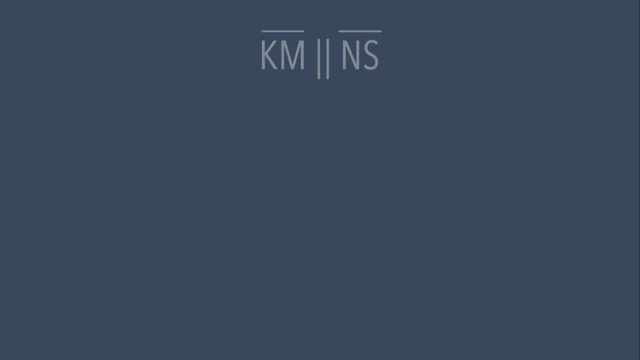 Let's try a different type of example. Draw and label the figure described. Line segment KM is parallel to line TF. First, we draw line segment KM Because we need the two line segments to be parallel. we need to make sure that the distance between them is the same. 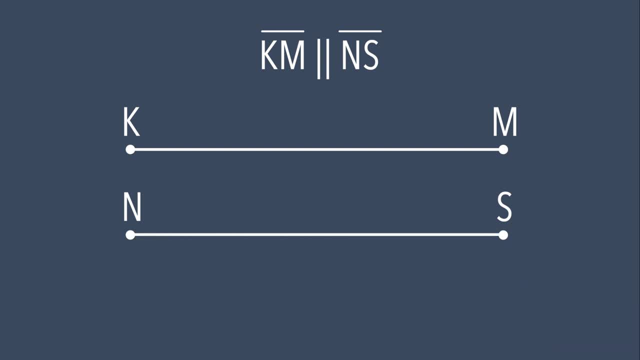 Now we can draw the second line, segment NS. As you can see, line segment KM is parallel to line segment NS, Because the distance between them is the same and they never intersect. Let's do another example. We need to draw ray MT intersecting ray UK at point S. First, 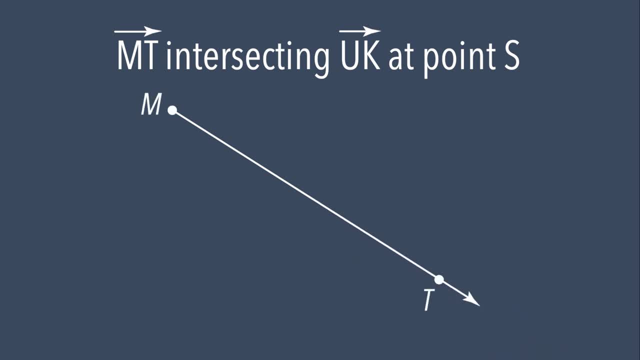 we draw ray MT. Now we draw ray UK. Now we draw ray MT. The point of intersection between the two rays is point S. Let's do another example. Line CD is perpendicular to line AB. Let's draw it out First. we draw line CD.